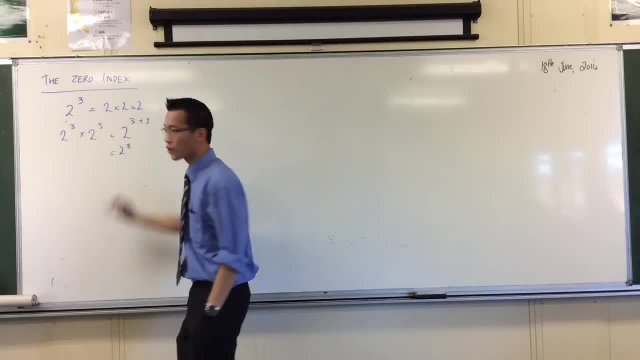 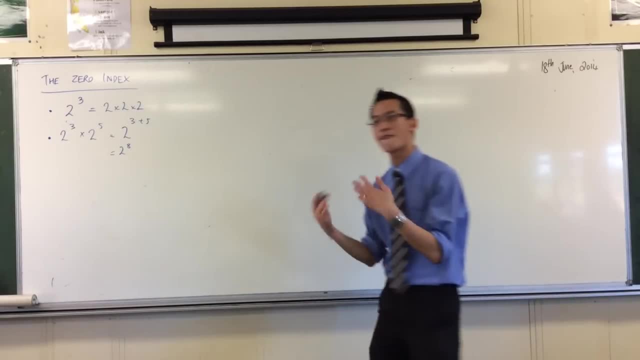 Okay, so it's 2 to the power of 8, good, So there's number 1, definition, number 2, multiplication. yesterday what you covered was division and it follows the same idea, but in reverse, right. 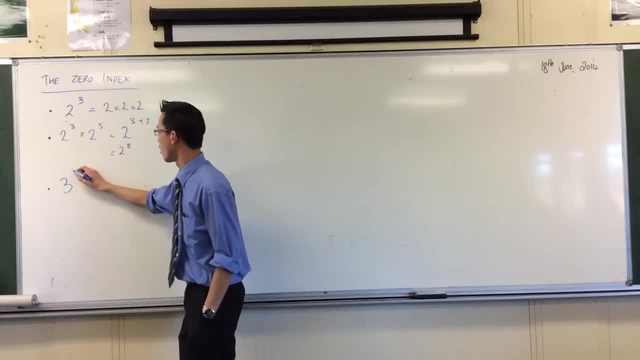 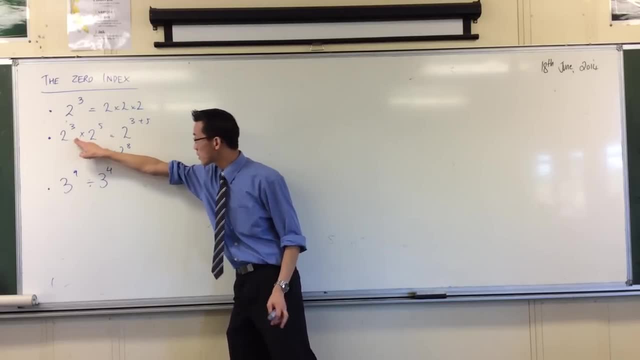 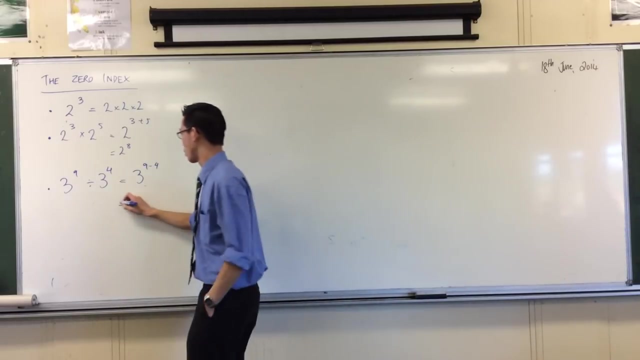 So if I had something like 3 to the power of 9, divided, Divided by 3, to the power of 4, okay, just like. yeah, just like. multiplication goes to addition here, division goes to subtraction, right, so you take away one index from the other, okay, so therefore, you get 3 to the power of 5, cool, okay. 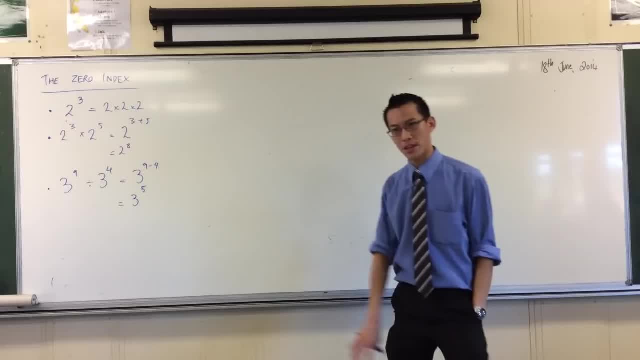 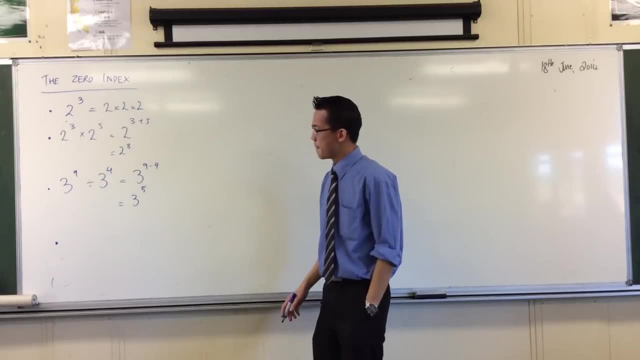 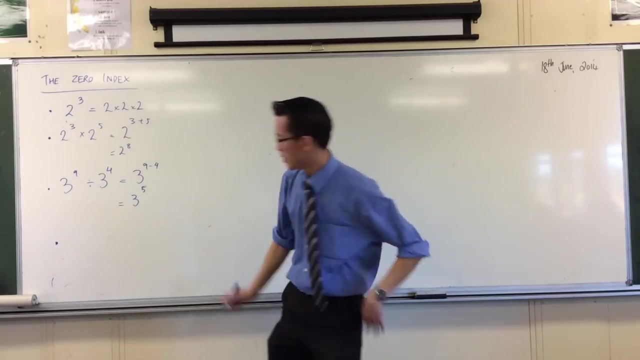 But we notice a few interesting things here, right? because if you follow this pattern through, we've done this with the table before, but now we can use this law. If you're like that, if I take, for example, let's now go. let's now go algebra. let's think about not just specific numbers, but any numbers we like. okay. 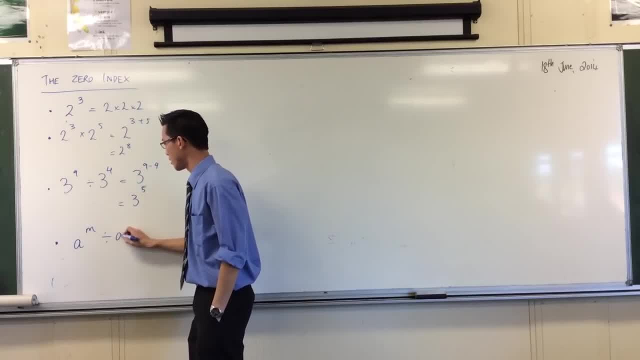 I think you might have remembered this. if you've got these two numbers, okay, so A, whatever it is any number you like, but the important thing is they're the same. And then you've got two numbers here, right, just following the pattern from this line. what happens? 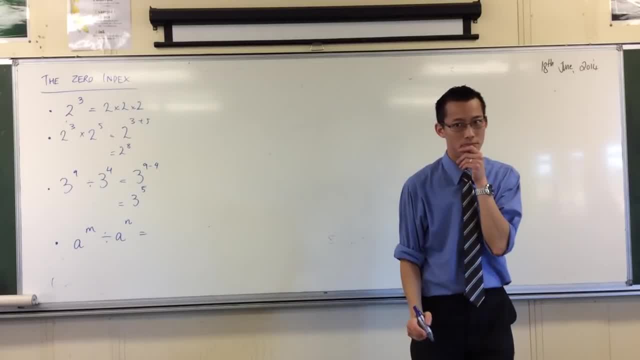 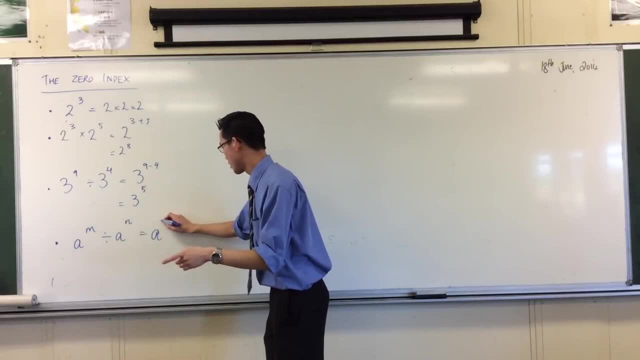 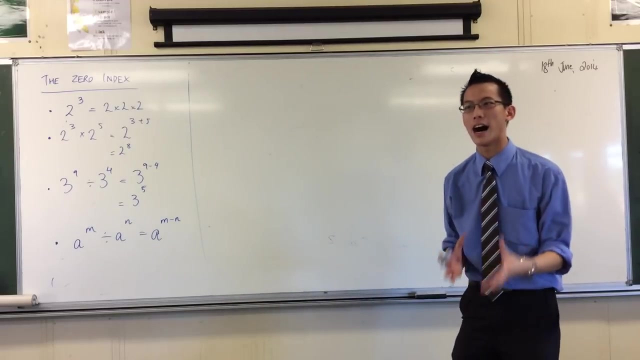 The base A. what happens to that? It stays the same right. and then, what do you do with the indices? Yep, good, okay, so this is what we've got, but now consider what happens if M and N are the same. okay, 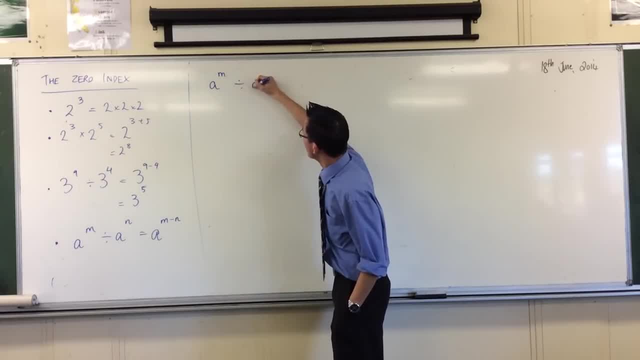 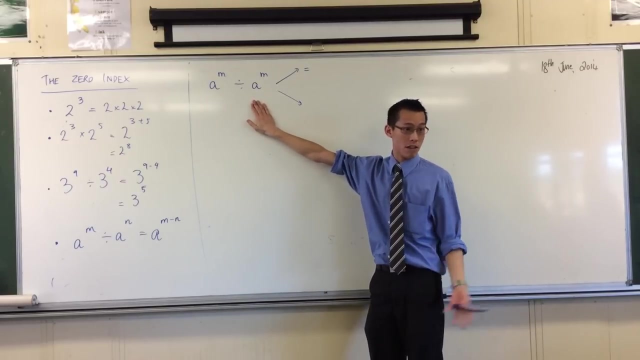 If I had this. good morning, welcome back to class, okay, great, alright, now, if the indices are the same, we've got two A's. So think about this right, two A's. you could say first look, it's a number divided by itself. right? what's a number? any number divided by itself. 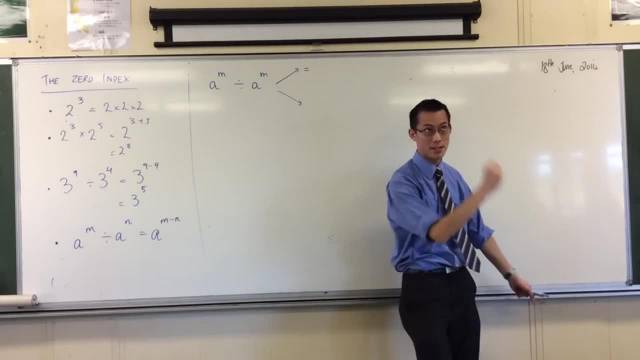 Divided by itself is one, like five divided by five is one and a hundred divided by a hundred is one. okay, so you can say it equals one. But in the same way you can follow this guy. see what happens. right, the bases are the same. so what happens to the base? 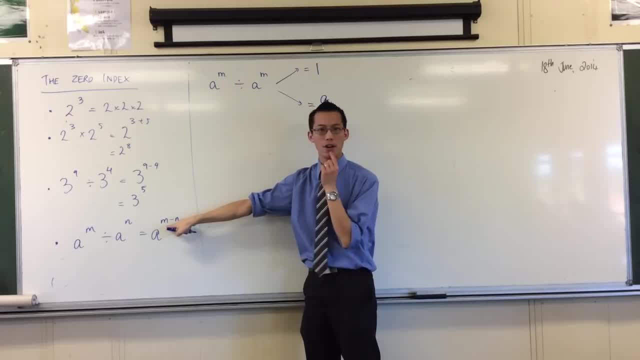 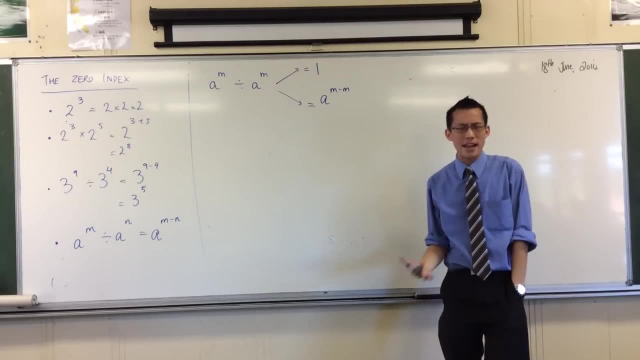 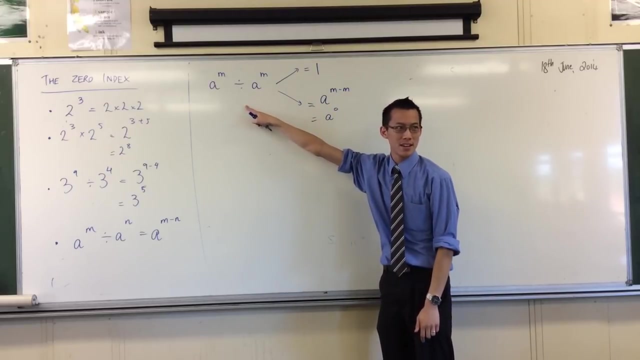 It just stays there, right? and then you go here, you go M minus. but both of the powers are the same, right. what's M minus M? A number? take away itself: it's zero, right, like five minus five is zero. three minus three is zero. so that's A to the power of naught, right, but these two things came from the same place, right? so that means they're the same as well. 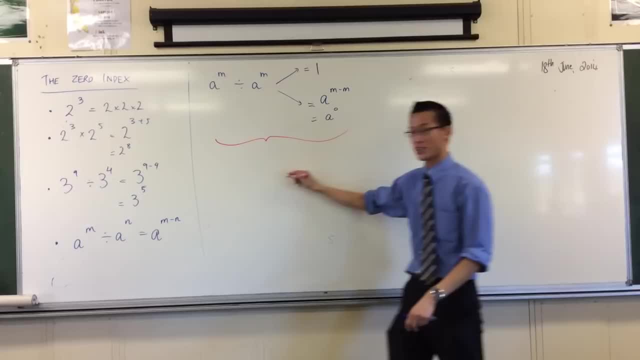 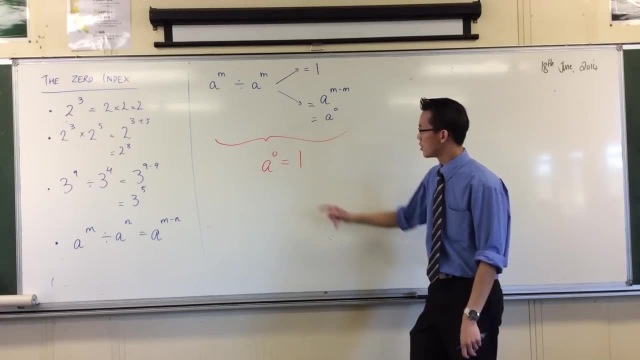 So that's the number zero, never zero. Yeah, that's right. So that's my conclusion. okay, what's your question? I thought I you just put A. you don't even put A to the power. would that be right if I just put A to the power of naught? 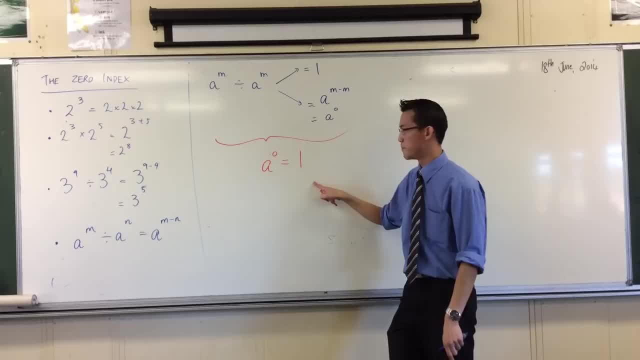 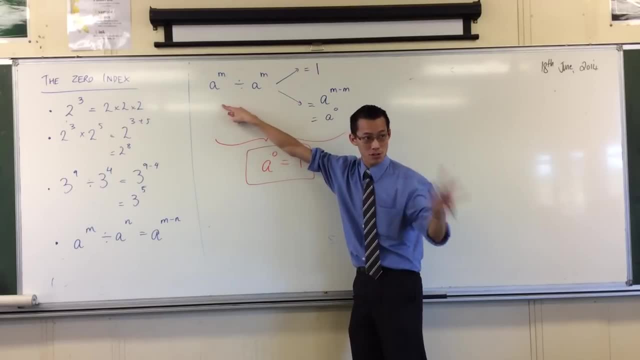 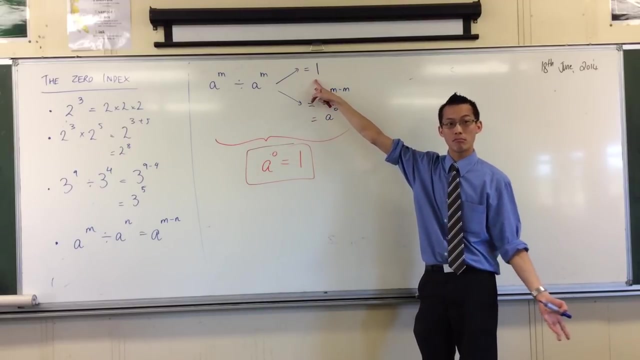 You mean A to the power of naught is A Yeah, just like A No. it's one. see, this is my point. okay, let me illustrate it to you again. I can think about this line here from two angles. I can say: it's just a number divided by itself, right, and whatever that number is, when you divide it by itself you just get one, okay. 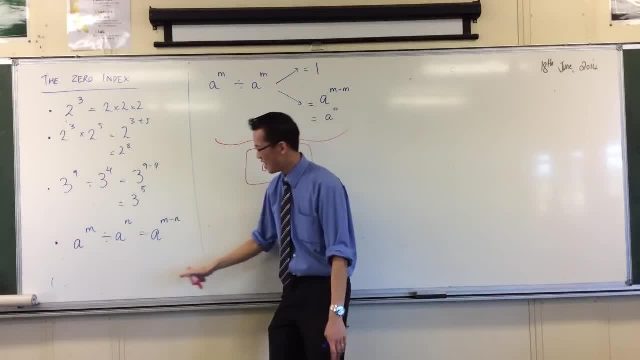 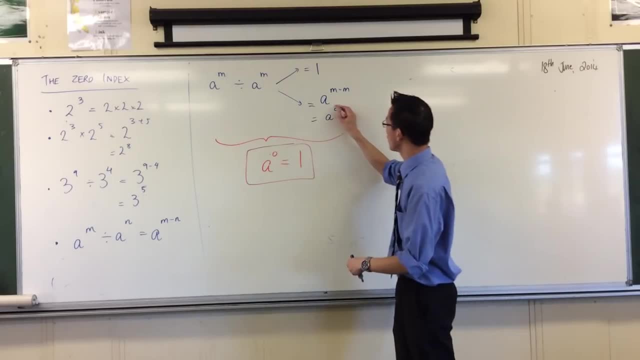 But alternatively, if I take what you guys learned yesterday: Okay, When you divide numbers at the same base, you subtract the indices, then this is what you get, okay. Well, if you go from the same thing and you get two different answers, that means the two answers are the same. okay. 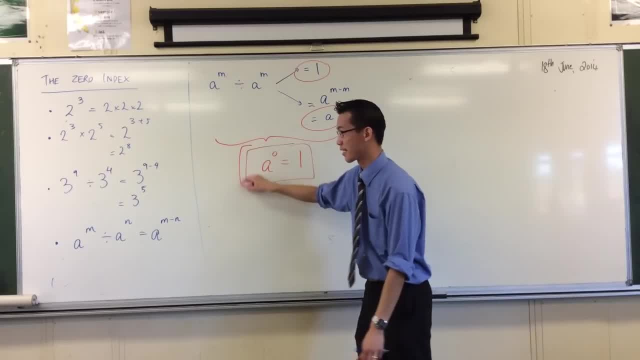 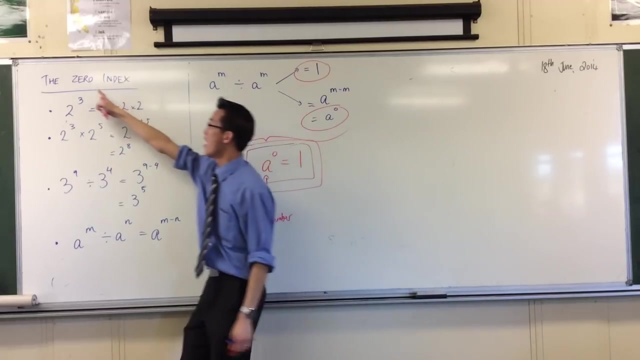 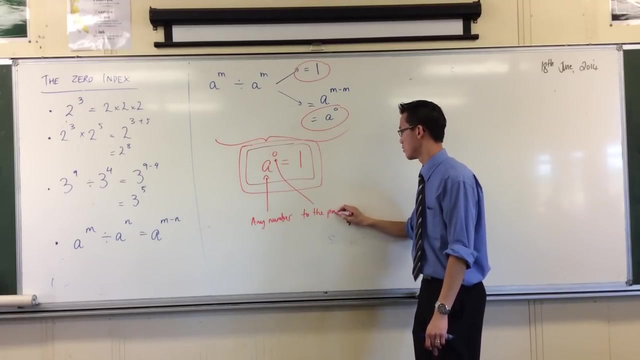 So that's why this is what you want to put in a big colourful box, okay. Okay, just go around the back That any number, any number there, any number- okay. if you raise it to the power of zero, if it has a zero index, okay. any number to the power of zero is one, okay. 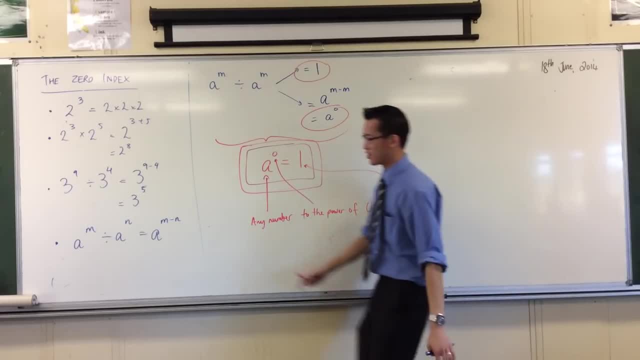 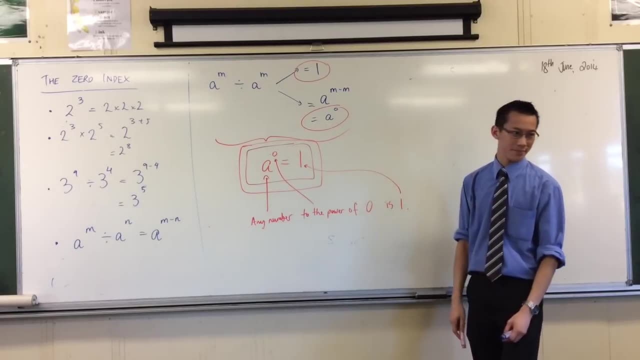 So this is, if you like. it's called an index law, just like all your other ones, okay, yeah. Yeah, it does look like A degrees Hold. on two different questions there. Firstly, it does look like a zero. 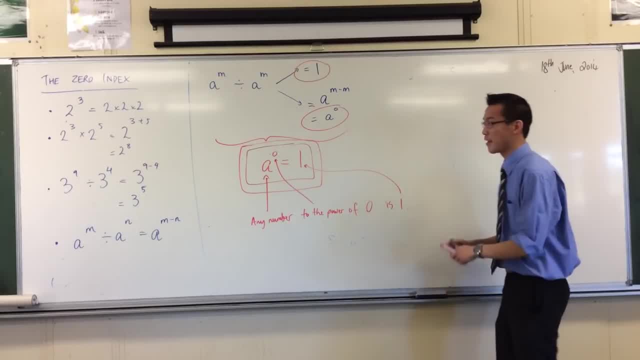 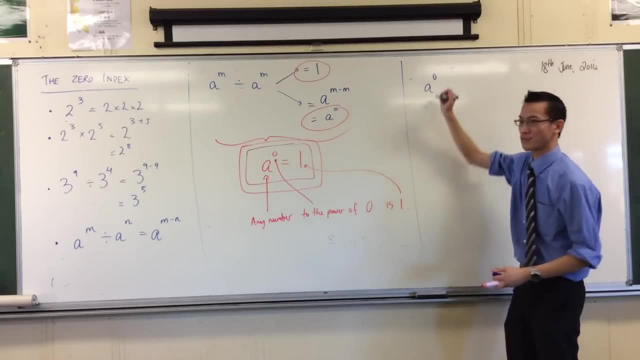 Sorry, like a degrees sign. There's not much way to avoid it. I mean, if I were to, if you actually typed it out. the very, very subtle difference is that if it's a zero it's slightly taller And a degrees sign is meant to be perfectly circular.